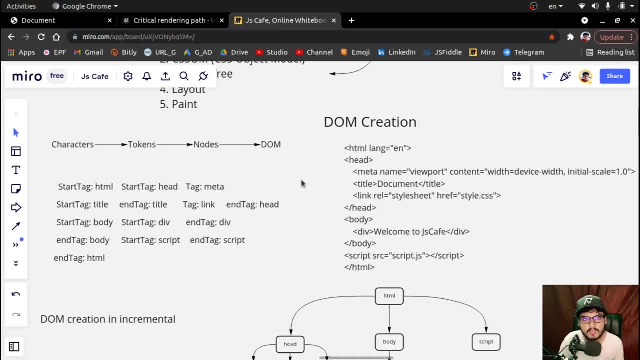 uh, if you have a look at the google's uh search page right, and whenever you type something and hit enter, you notice that uh, the head section of the page right, uh, the part where uh there is google's logo, where there is uh navigation links, uh, you know, map, map, images, news, etc. that part is: 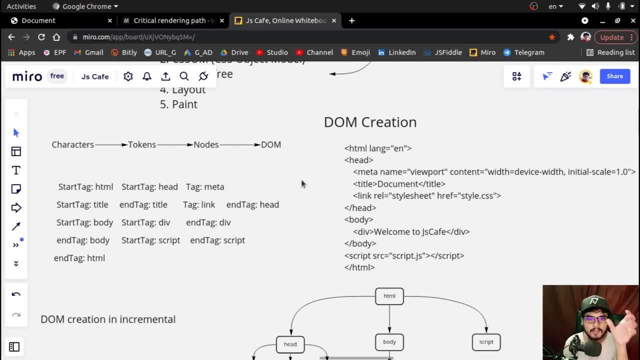 actually loaded first and followed by that, you see that the search result page are page are rendered. okay, what i mean by that is the dom can be, you know, created incrementally. let's suppose you send one, some part of the html, uh, in one request and another part of the html in another request, right? and what browser will? 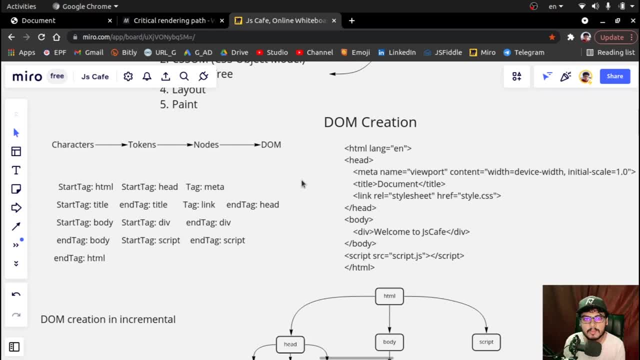 do is browser can incrementally add those uh dom, uh structure and it can render it on the screen okay, so it's not like it has to finish all the dom creation at one go. if you supply some more html to the part of the uh you know uh process, then definitely that would become a part of the dom. 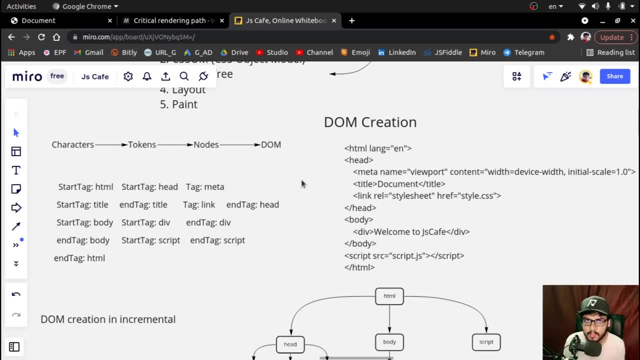 tree. okay, this is why the uh dom trees are incremental. and what next is that? uh? token creation. right, so this is uh. these four are the steps, basically, that is involved in the creation of the dom and that is uh, characters, tokens, nodes and dom. okay, for example, i have taken this small: 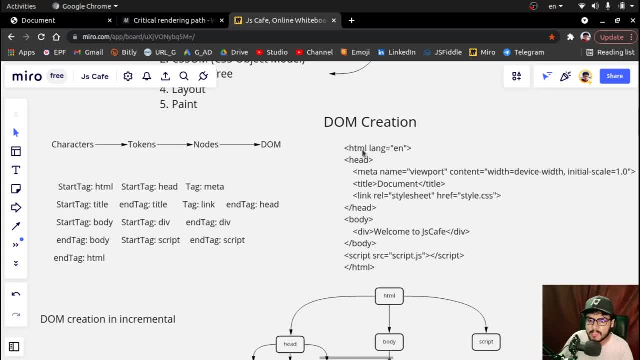 code snippet: uh for html and i have taken this code snippet for html. and i have taken this code snippet: uh for html and i have taken this code snippet for html. we have a html tag: head tag, meta title, link uh. closing height, tag, body uh. div tag with some text and closing body and followed by script tag. 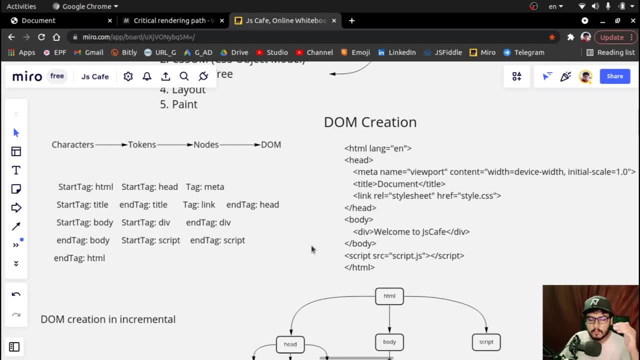 and, finally, we close the html. so now, when the browser starts, you know uh going through these um quotes, what it does is it uh creates a token for them. okay, so for uh browser, these are the characters. okay, these are characters, and what it does is it creates a token out of them. so 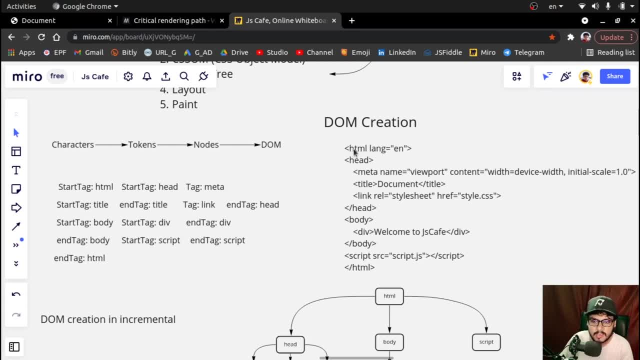 what tokens look like is that we start with HTML, so it will assign a token saying it is a start tag. okay, start tag is basically a token. then we come to head tag, so again a token will be created- start tag- with value head. okay, and we have a meta tag, since meta. 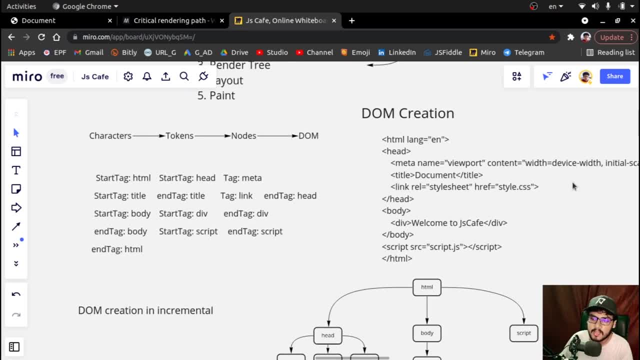 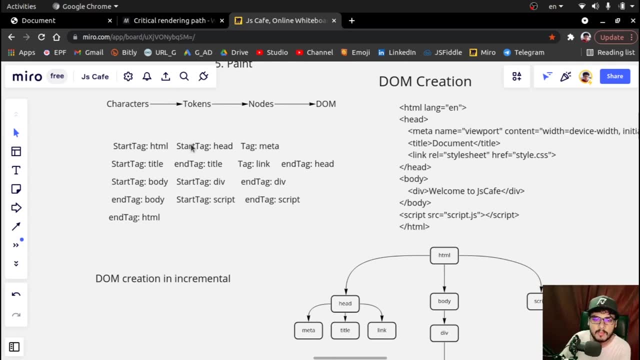 tag is self-closing, so it is a self-closing right. so it doesn't has the ending tag, right? so so we have changed the name of the token from start tag to just tag only. okay, it is meta. then again, we have a title, so it is a closing tag, so we have a start tag title and. 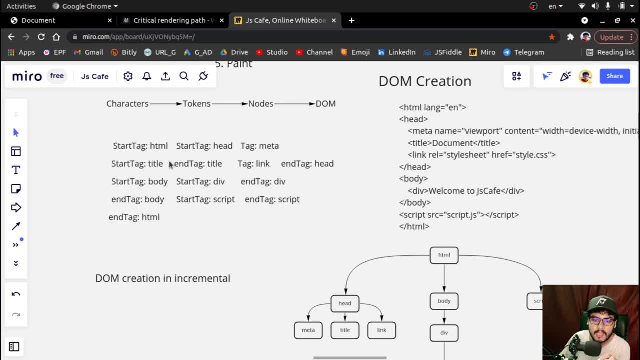 end tag title. okay, so whenever HTML, you know, tag- ends, we give a token of end tag, and if it is a self-closing then we give it a token of tag, and if it is the opening tag then we give it a token of start tag. okay, this is the nomenclature and followed by link. link is, you know, self-closing we have. 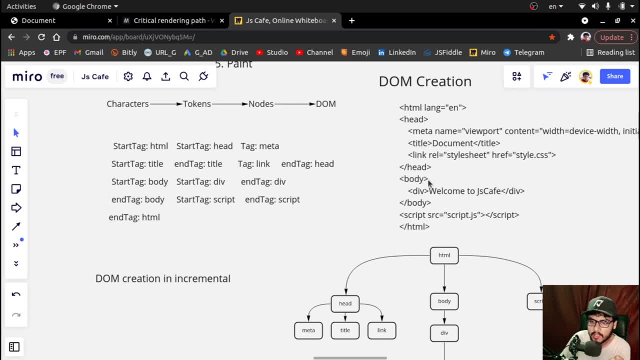 a tag, then we close the head. so we have an end tag with a head. we have a start tag of body. okay, we start tag of div, end tag div. we have end tag body, we have a start tag script, we have end tag script and we have end tag HTML. so this is how the tokens are basically. 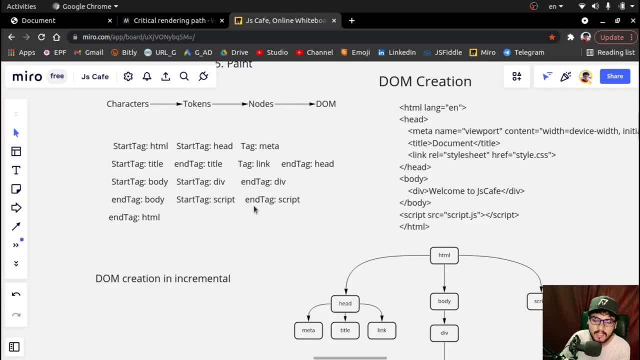 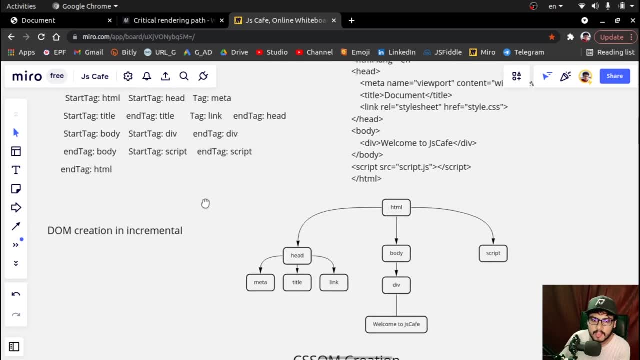 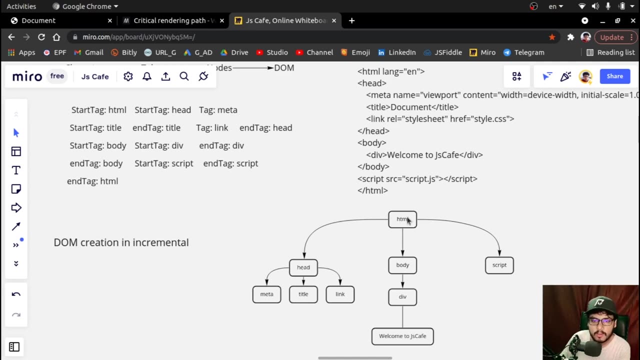 generally created. now, once these tokens are created, what you know a browser does is it converts them into nodes, something like this: okay, so it treats a node whenever there is a start tag- okay, or tag, and it creates a node. and if there is another start tag followed by a start tag, then this means that there is one node inside. 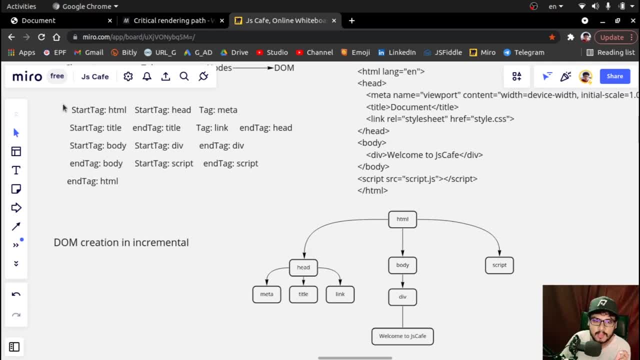 a node. okay, so we see that a head was inside this HTML, so we created a head again. we saw a tag inside this start tag only so this meta came here again. we saw title, so title came here. we saw link: link came here and finally, when head was closed, then browser came to know that there. 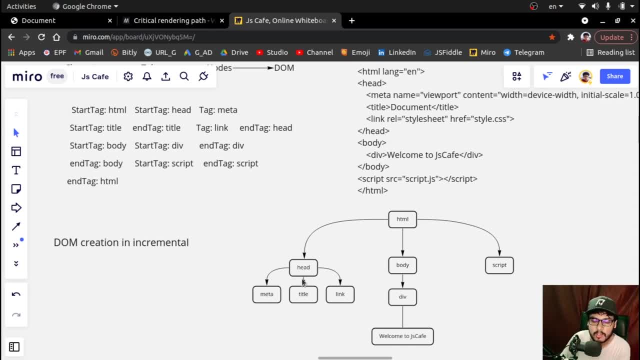 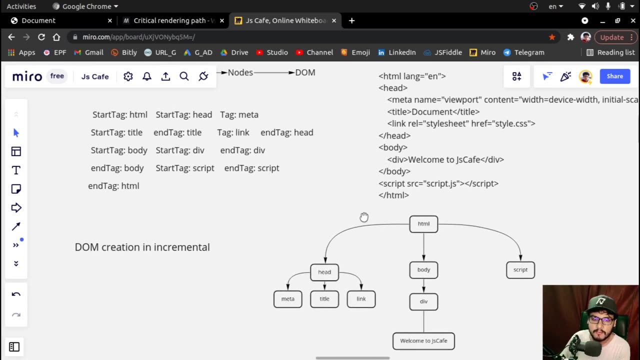 is nothing else remaining inside this particular node. these are the only children. okay, then it comes to body. then again, it comes to body, then it creates a div and it assigns a text. okay, so this is how this DOM tree is created: with the help of tokens. right, if you are a? 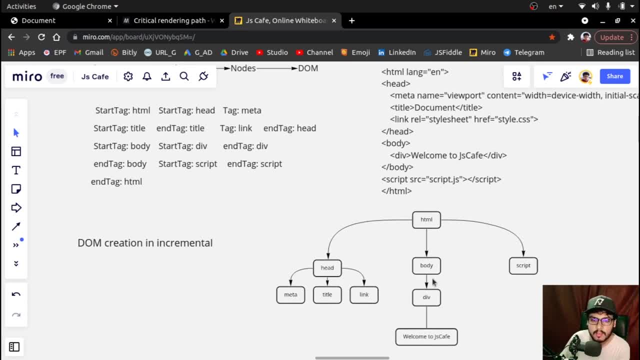 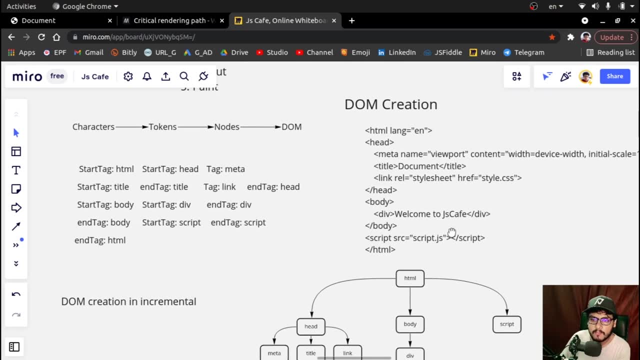 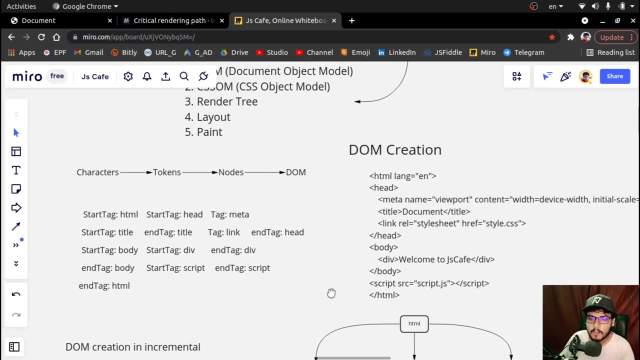 dad and do pause the video. run through these tokens and try to match if they, if you are able to form this particular tree, right? so this is the part where that DOM creation is happening and I have explained how the tokens are created. okay, so once this tokenization, 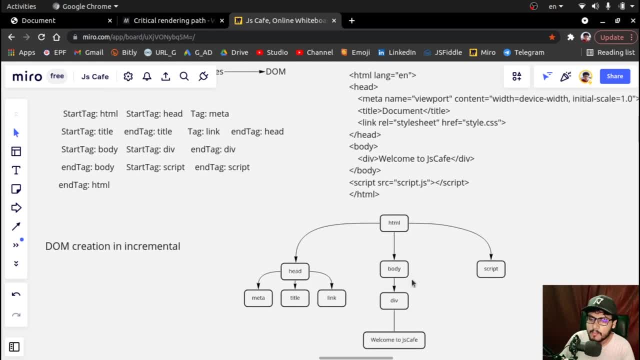 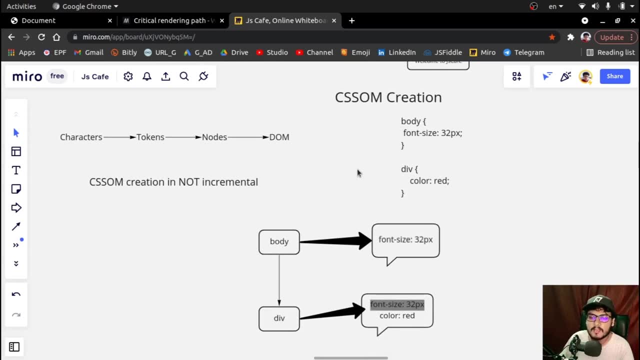 is done and we have a DOM ready. okay, so Dom basically has everything. okay, every tag. now we come to the creation of CSS. okay, CSS object model. okay, CSS object model. okay, I have created. so what is happening is we are having: we load when we load our css files. okay, so, uh, again these. 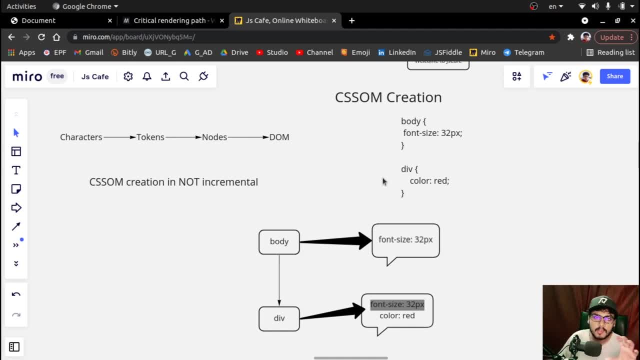 css file is again converted into a- you know, object model- okay, a tree like structure, and again the process is same: characters, tokens, nodes and dom- okay. so this is how the process of css om is created. for css, the tokenization and the character identification is a pretty different. they have 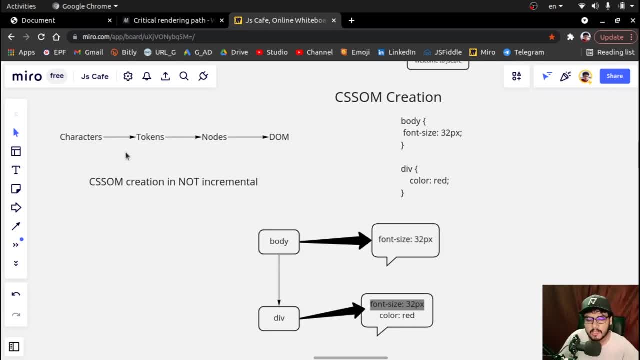 their own logic, and discussing that particular logic is, uh, not necessary at all. if you are really interested, then you can- uh you know- search for how- uh you know- css particularly creates a dom. uh you know tokenization and other stuff, but at this point, uh, it doesn't really matters, okay. 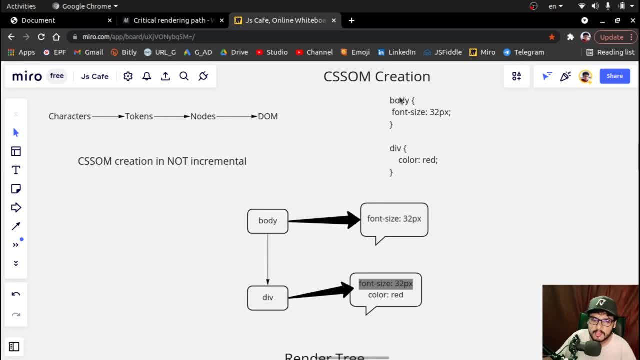 so what matters is that you uh- let's suppose you you have these tokens, okay, uh, body and div, you uh give them. uh, you know, you generate the tokens and, based upon that token set, you generate this particular tree. right body, we have a body uh node and in inside a body node, we have a div node. okay, but apart from uh these, 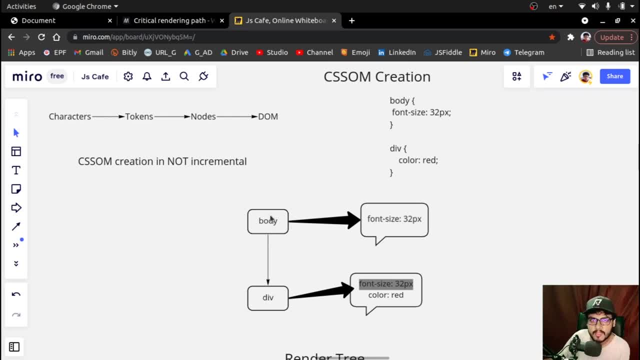 nodes. these nodes are attached with certain properties. okay, the properties are what lies within these curly braces. okay, like, the body has a font size of 32 pixels, so this property is associated with this particular node. now, when we cascade down to a particular child, all the property that the parent has is cascaded down. 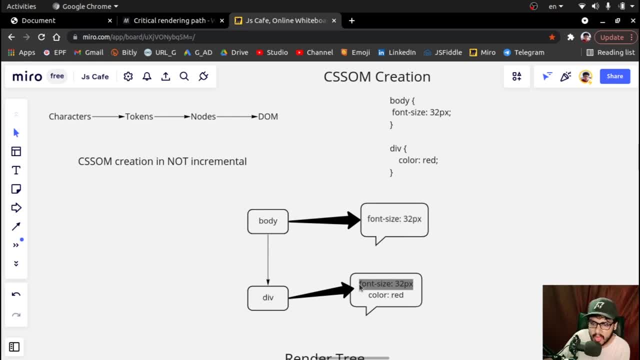 okay, so i have marked this font size, 32 pixel, as a gray area stating that this property is cascaded down from its parent. okay, and we see that this particular div has its own property that is color red, so i have written this color red property as well. okay, so this is why css is known as. 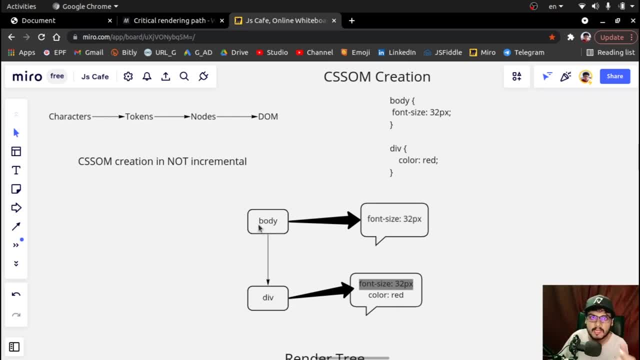 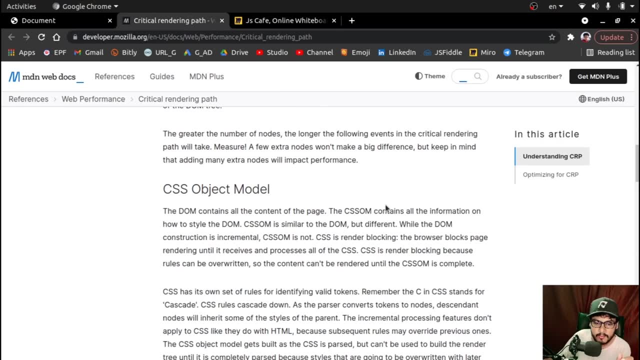 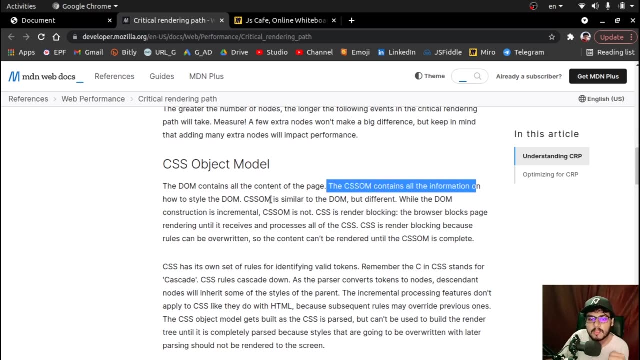 cascading style. she's right, because we cascade down the styles to, uh, children from their parent, right? so this is the css on creation. okay, so let me take you to css on. so the dom contains all the content of the page and the css form contains all the information on how to style. 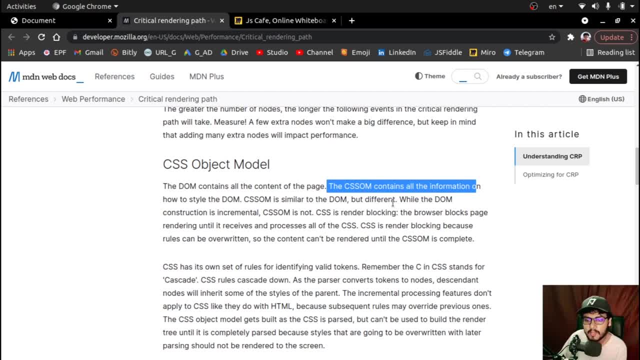 the doms. okay, css is similar to the dom but different. okay, while the dom construction is incremental, css arm is not okay. css is render blocking. the browser blocks the page render until it receives and processes all the css. css is render blocking because rules can be overwritten. 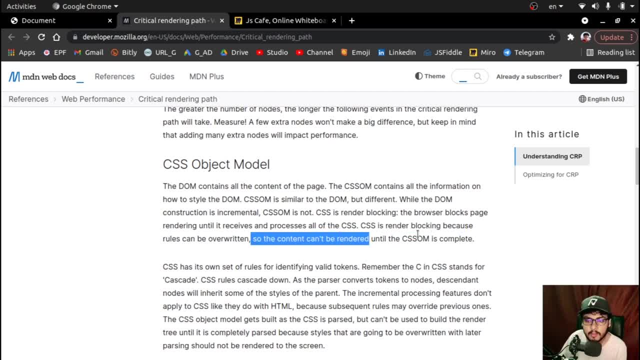 the content can't be rendered until css is almost complete. okay, so what does it mean? so we saw that the dom creation was incremental. right, like we discussed that we can pass uh html at later part of time and they can be a part of the dom, but this is not with css. 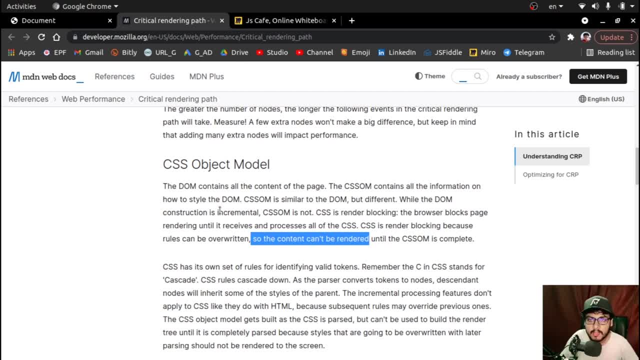 okay, css, almost con, is not incremental, it has to be computed once at all. okay it, it will be computed once. only the reason is that there there are chances that at the later point of stage, uh, the css styles can be overwritten and this will again trigger a repaint, or 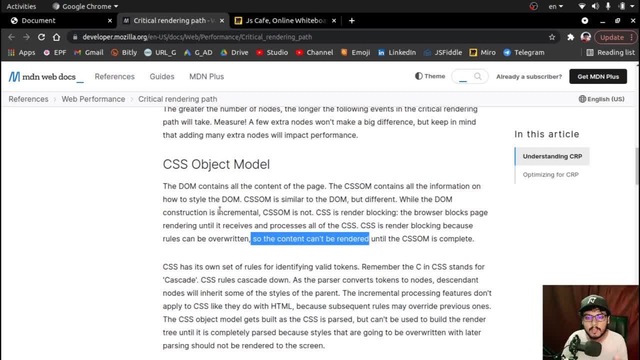 uh, you know layouting, okay, i'll tell you uh what painting and layouting is done, but for now, remember that in order to avoid uh layout and painting, uh, that is that is why css arm is not incremental and the all of the construction is basically: uh happened when it start parsing those. 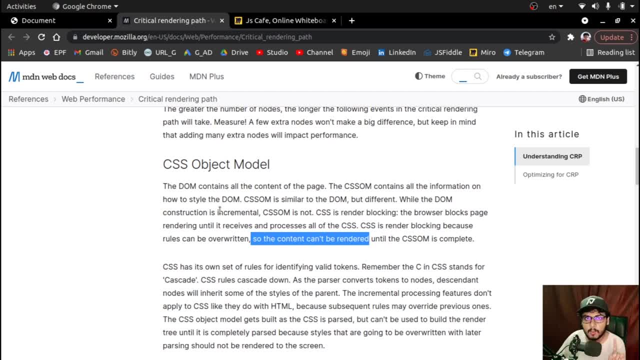 css files. okay, so css is constructed once only. okay, so it is incremental. and again, yeah, uh, to compare, uh, you know, javascript has ability to alter our styles, right, uh, so again, we can alter our styles. but that is true javascript, but while parsing a css file for that particular time. 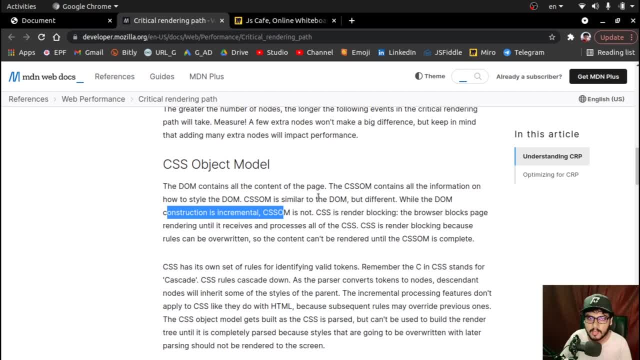 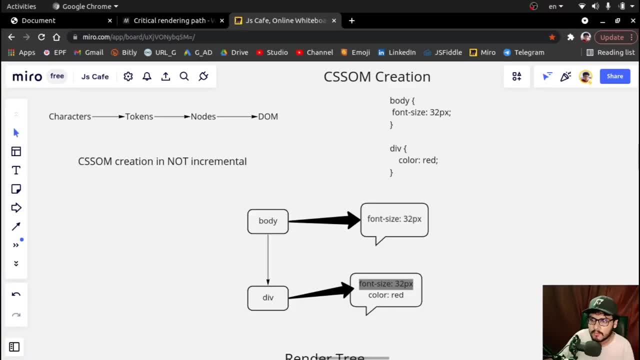 we? uh create our css on at once, at one go only? okay, that is one thing we have to note about. so css, when css arm seems is created, uh, when we we see that we come to this part that is gender tree. so when we combine dom and css arm together, then we get p? umand готов to stay. so we gotta identify uh? d. or when we we see that we come to this part, that is mandatory. so when we combine dom and css arm together, we can specify- let's specify path item between each of these when cssarlo om is created and ever applying the fös into the tile to be able to re-bonnet, let's see how you? you know that font size is different in the parsley, so first let's. 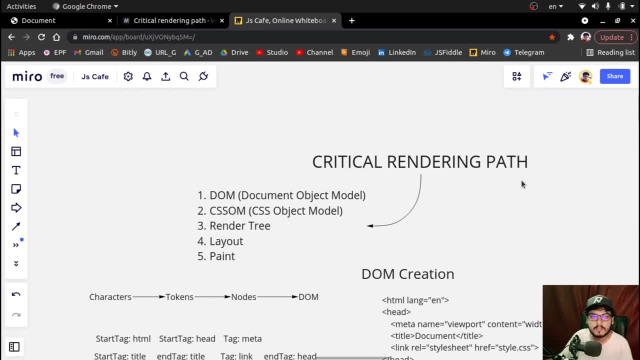 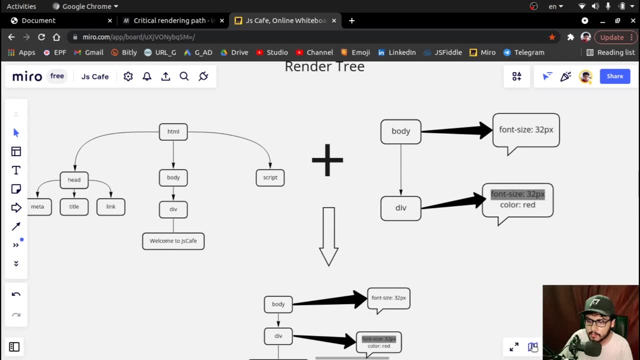 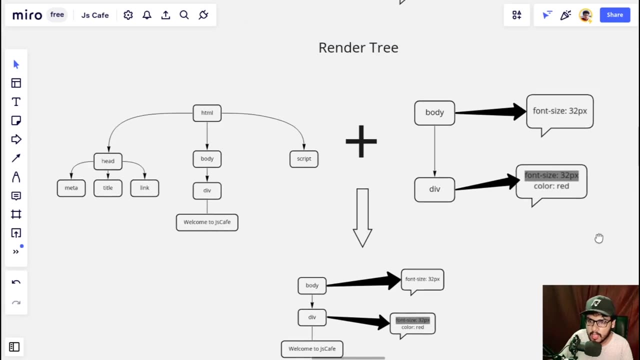 we generate the render tree and that is actually what is visible on the- uh, you know our screens. so if you come have a look at this diagram, i'll zoom in a little bit, okay? so if you look at this, this is a render tree and in this render tree you see, on the left hand side, we have this particular 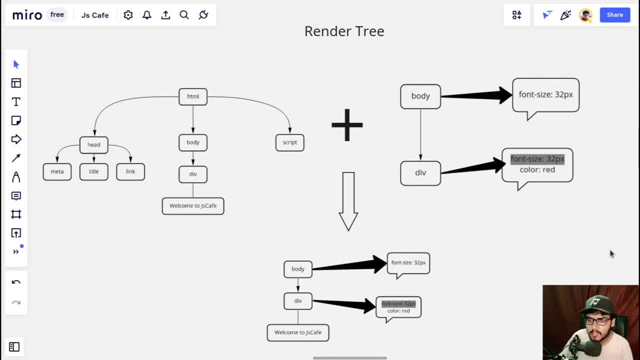 dom, which we just discussed above, and on the right hand side we have this particular css orb. when we combine these two, we generate our render tree. so render tree may, the things are only contained which are actually visible on the screen, so anything that doesn't contribute to. 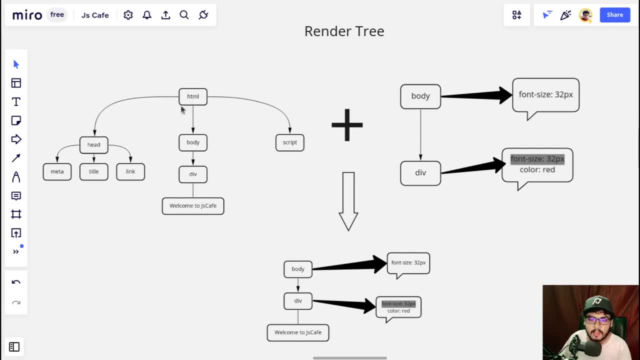 uh, you know, to adding the pixels is not added. okay, so whatever is present in this head, it is omitted. whatever this html tag is also not contributing, so this is omitted. this script is also not contributing, so it is omitted. so only part that we take out of. 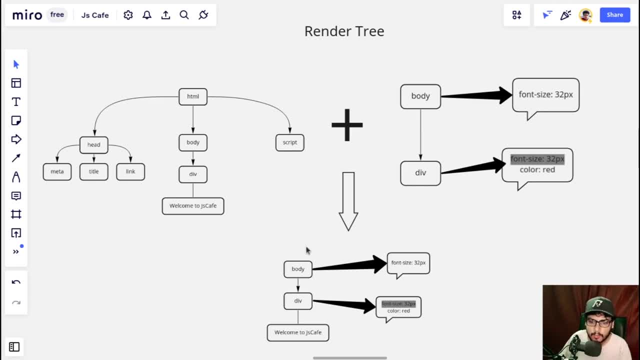 front end is not contributing, so this is omitted. so only part that we take out of front end is from the dom. is this body part? okay, so we take this body part, we add it over here and whenever we start mapping these nodes, okay, we map body with body, we map div with div. we found that these were: 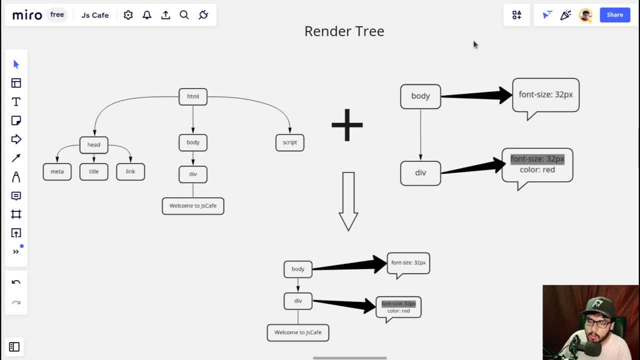 the properties that were associated in the css arm. so we took those properties and applied them in this, okay, in these, in the render tree. so this, this is how what uh, render tree looks like and this is what exactly is rendered on your screens. okay, so so up till now, we have discussed dom creation, we have discussed css on creation. we have 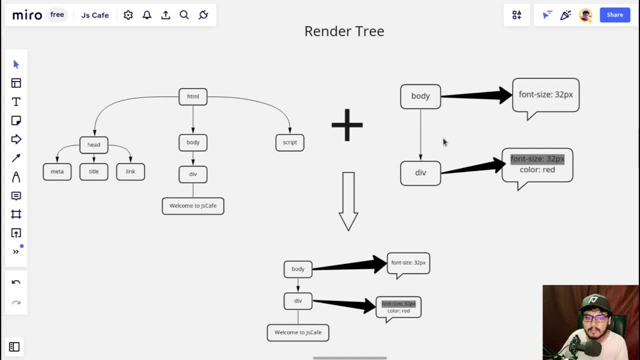 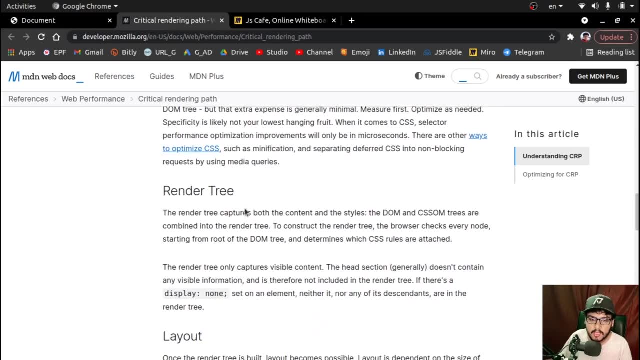 discussed render tree and when this render tree is done, then comes the layout and painting. okay, uh, i will take you through this uh render tree. so render tree captures both contents of uh content and the style. the dom and the css songs are combined together to form a 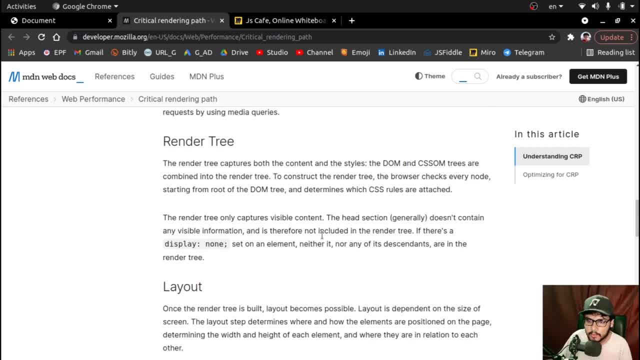 render tree. okay, this is as simple as that. and one thing to note that is, if there is any content that is set to display none, then that particular node will be omitted from the render tree, although it will be part of the dom, but it is not part of the render tree. okay, that? 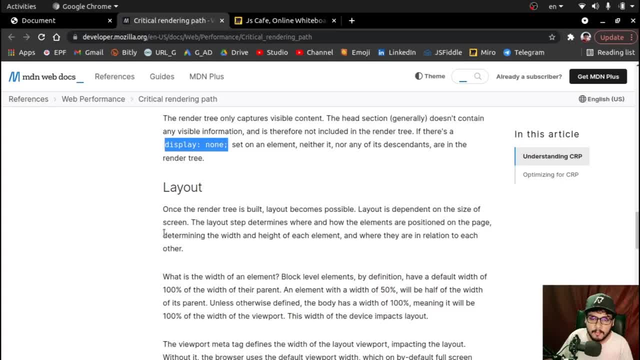 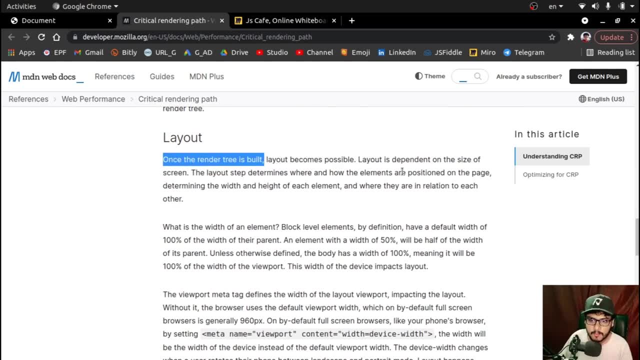 is one. uh, catch here. okay, now coming to layout. so layout is nothing. uh, basically, layout is like: once the render tree is built, layout becomes possible. layout is dependent upon the size of the screen. the layout step determines where and how the elements are positioned on the page. 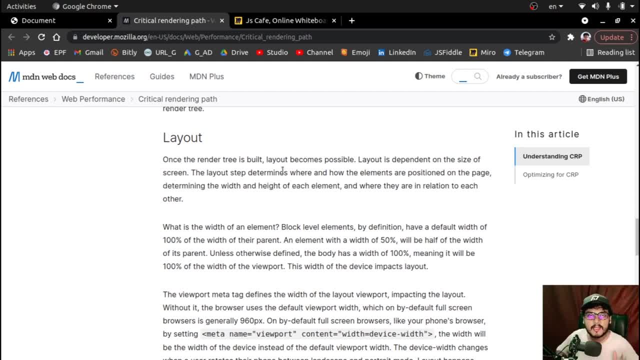 the width and height of each element. okay, so layouting is kind, of, you know, calculation phase for uh, you know for the for the crp process. by calculation phase i mean that, uh, when, once you have all the uh nodes of the render tree present now browser does is that it identifies that oh, 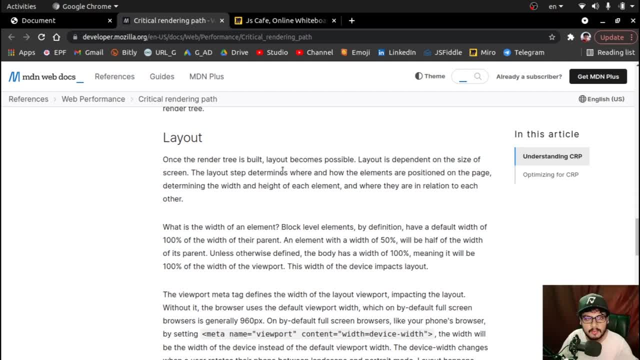 this is a body. so according to these properties of css on, and according to these properties of you know, uh, dom, uh, this would be the height and weight of this particular node. now i traverse a one step down. okay, now comes the sum. for example: div tag, div node: okay, 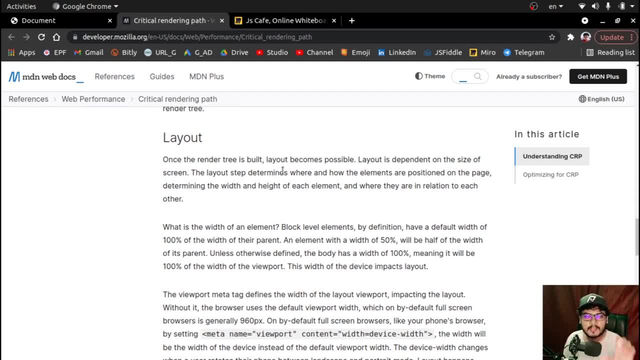 so div may. it calculates the height and weight via the css on properties and it also checks the attributes or particular, uh, you know, via the dom and again it computes. okay, so this would be the height and width of the this particular div tag. okay, and this um steps is repeated until: 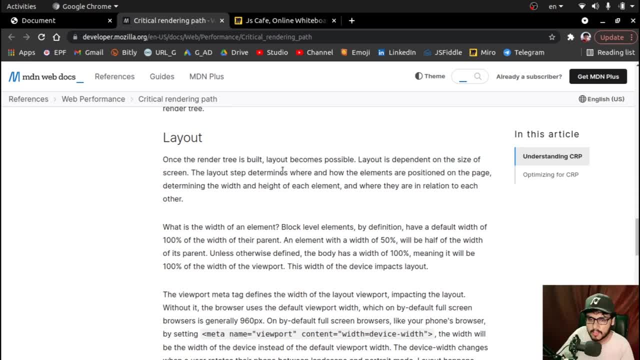 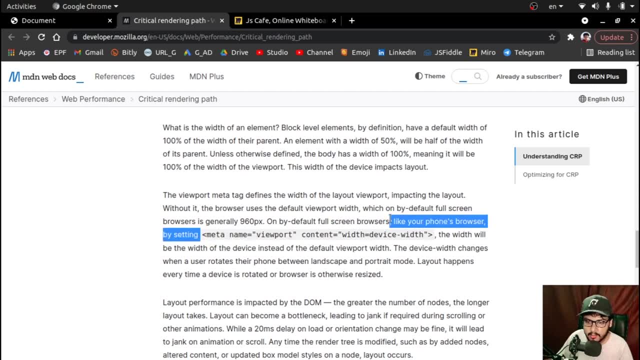 unless we traverse our whole rendering tree tree. okay, so this is the layouting step and in this part, uh it it talks about this meta tag. okay, so by do it is saying that by default, full screen browser is generally 960 pixels. one on by default full screen browsers, like your phone browser, by setting meta tag name: viewport. 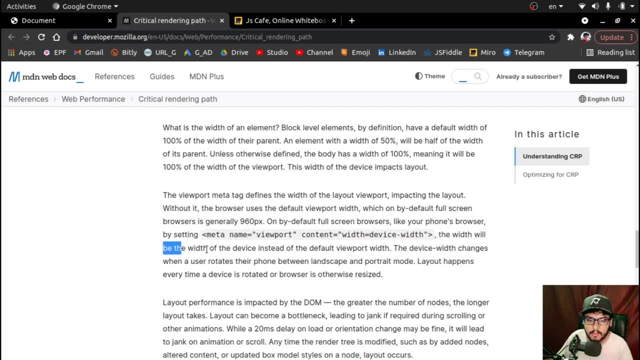 content: full device width. so the width will be the width of the device being used, of the default viewport. okay, so adding this particular tag is really important if you want the viewport to be the full width of the device on which you are actually seeing. if you don't do this, then by 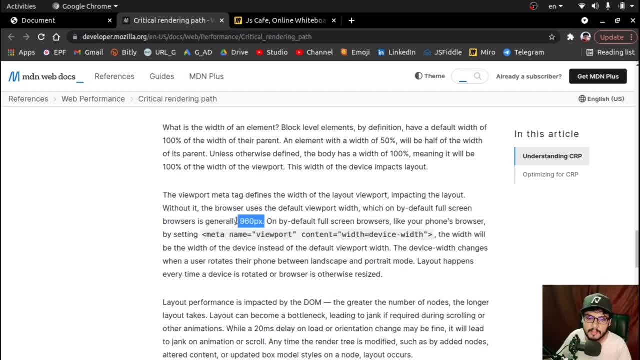 default, the- uh, you know size would be 960 pixels. okay, so this would, you know, this would hamper, you know, the layouting phase. okay so, uh, let's suppose you are not uh, putting this tag uh into your uh. uh, you know html and you are setting. 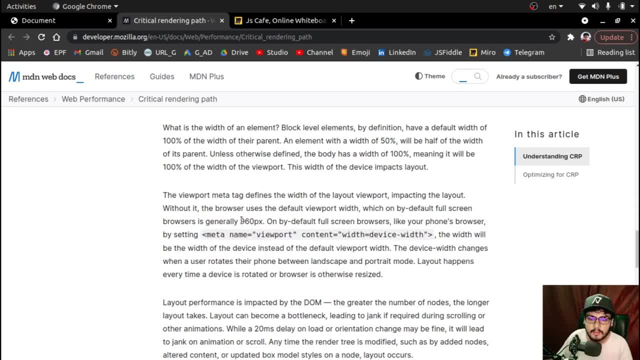 a div to a width of 100. so this would be. the 100 would be equal to 960 pixels. okay, but if you, if suppose you are on a shorter weight, for example, 320 pixels, okay. now you don't want your dev tag to be 960 pixels. instead, your viewports, uh, you know which should be 320 pixels. that should be. 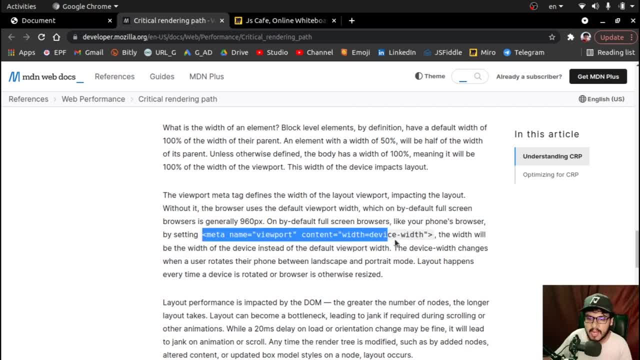 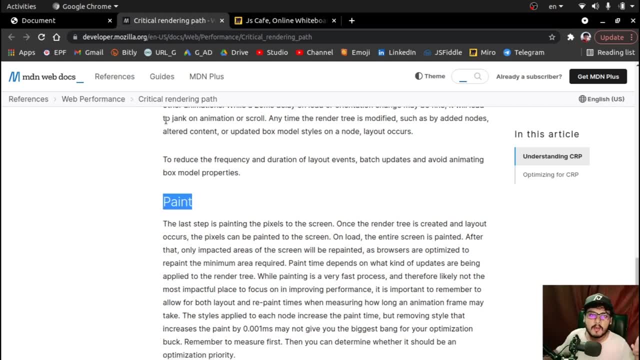 of your device, okay, so it's very crucial for you to add these properties, um. in those now comes the painting part. the painting part is the simplest one. once you have all the computations ready, you know how much width and height you want to assign to a particular node. 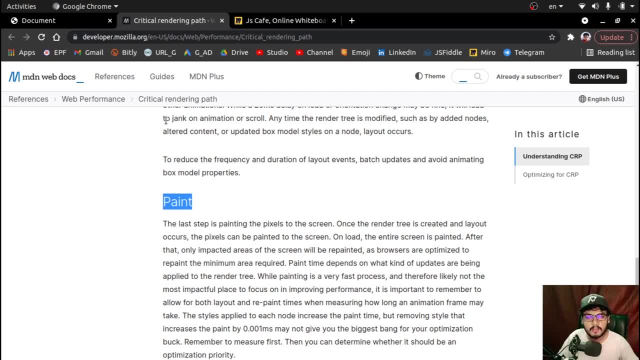 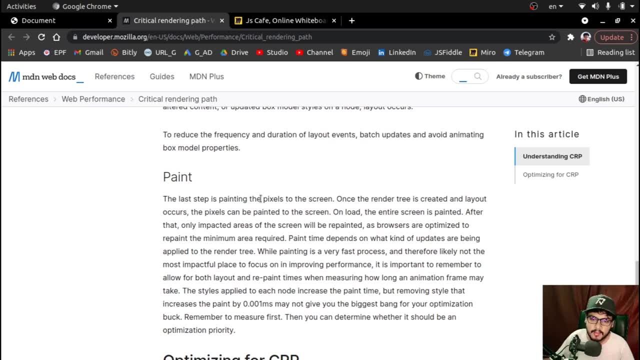 now browser does that is it just paints them on the screen via the help of pixels. okay, so this, uh, let me read this out for you. the last step is painting the pixels to the screen. once the render tree is created and the layout occurs, the pixels can be painted on the screen. 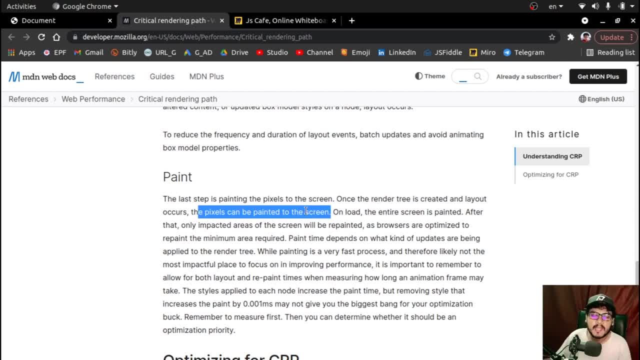 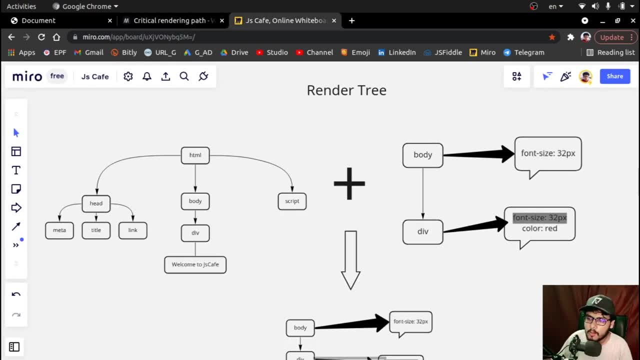 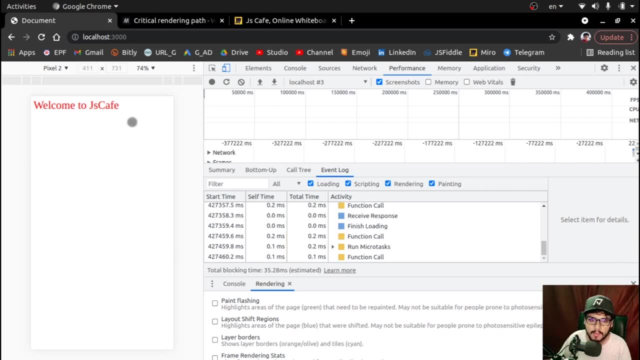 okay, this is very simple step. it's just that, uh, painting is like, uh, you are uh seeing the things on your screen now. okay, so these were all the five steps, um, of uh, critical rendering path. and uh, yeah. and also, uh, i have a small code snippet, uh, ready for you. uh, to show you how we. 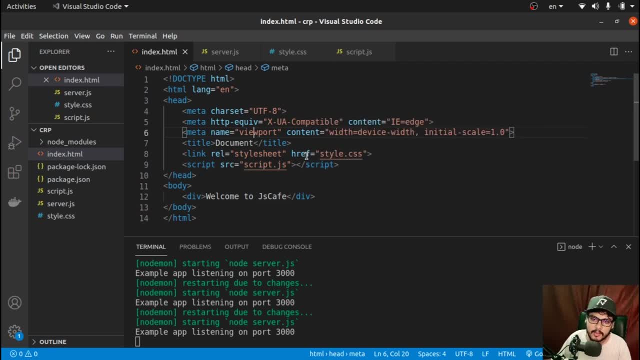 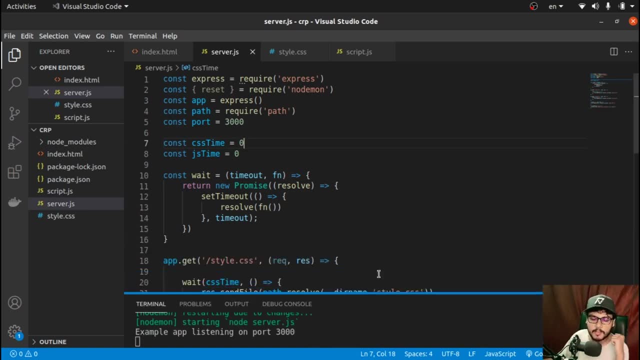 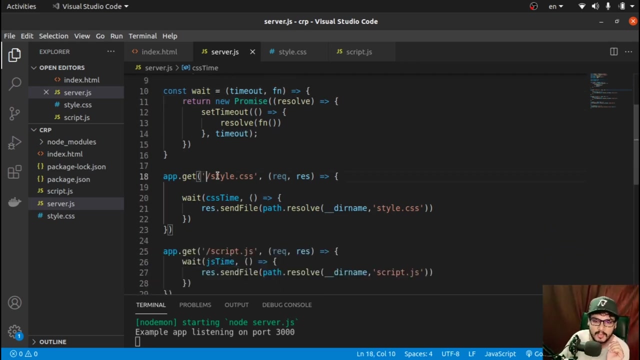 can actually see these steps, uh, in your, uh, you know, um in your dev tools. so i'll tell you how the setup i have done, the setup up till now, and what's the agenda of this particular setup. so i have created us a basic express server, node server right over here with me where i am serving a style. 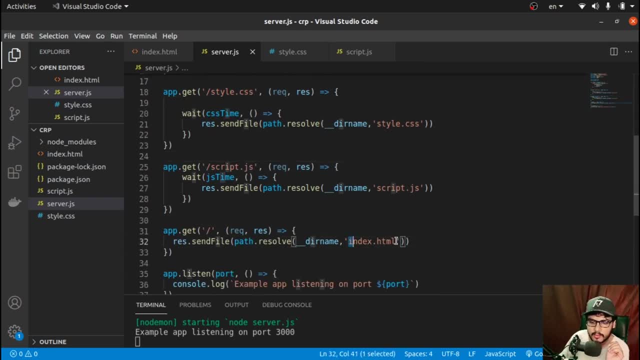 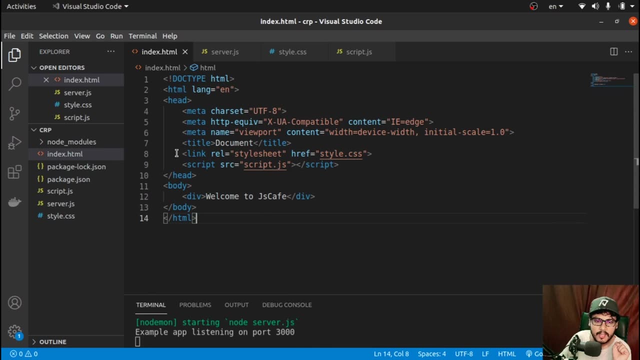 dot css, scriptjs and indexhtml file from this part, and my indexhtml is something what it looks like this: it has a style sheet, it has a script tag, it has, um you know, a div tag and something else. so, uh, let me uh put this script tag uh at bottom for this example, particular example. 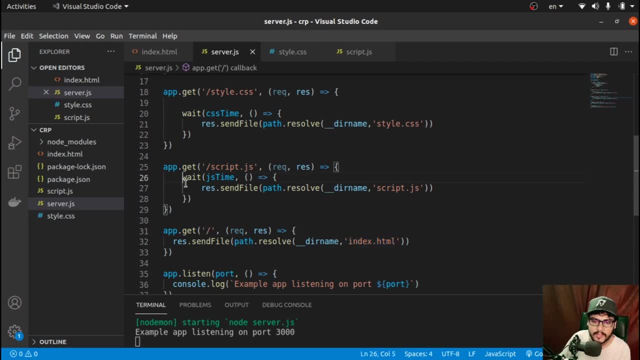 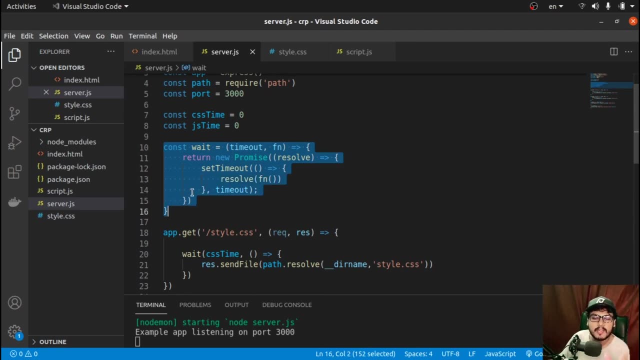 and yeah, and we have a weight. i have created a weight function over here. this is just to add, you know, to add a delay on sending some files. let's suppose someone creates a very heavy css file and it took, uh, five seconds to load right. so just to. 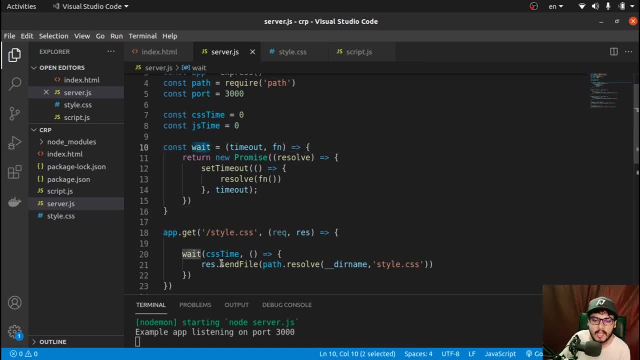 mimic that experience, i have created this a weight function and so that whenever i change this- uh you know, time, uh the load time of these files, i can, you know, show you how uh this ss is uh render blocking, how this js is render blocking. okay, so just wanted to show you those. 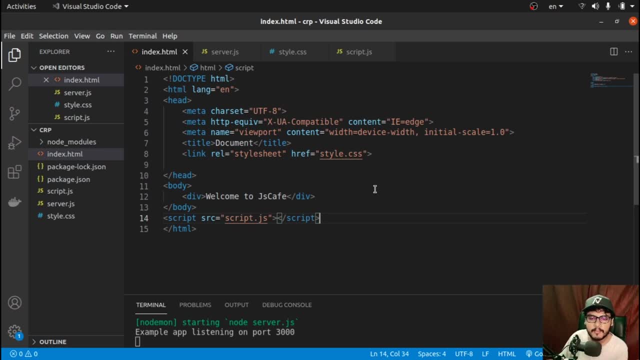 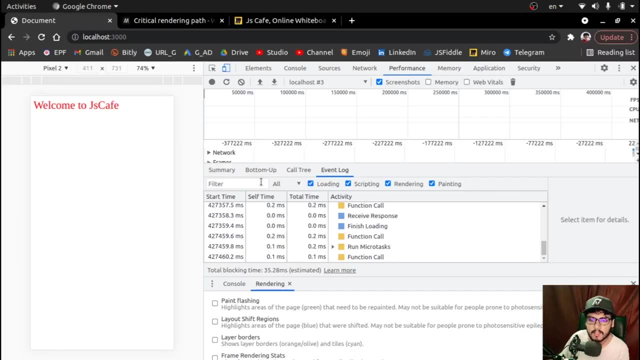 stuffs. so, but before uh showing that stuff, let me uh show you the uh critical landing path, lifecycle methods, uh onto your dev tools. okay, let me uh hard reload this once. okay, and what i'll do is i'll do ctrl shift, e to record it. wait. 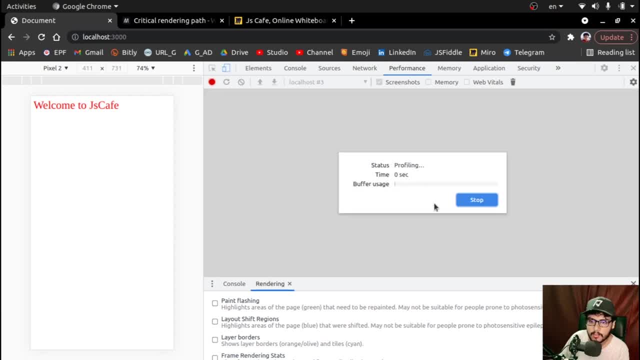 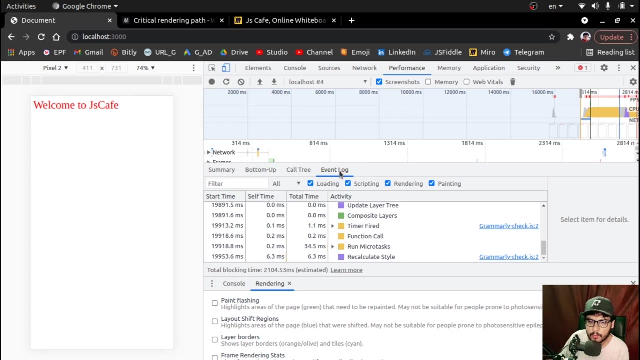 uh, let me record this up. okay, uh, let me record, stop, yeah. so if you go to the performance tab of your dev tools and go to event logs, make sure all these boxes are checked. and if you have a look at these steps, uh, let's have a look at them one by one. 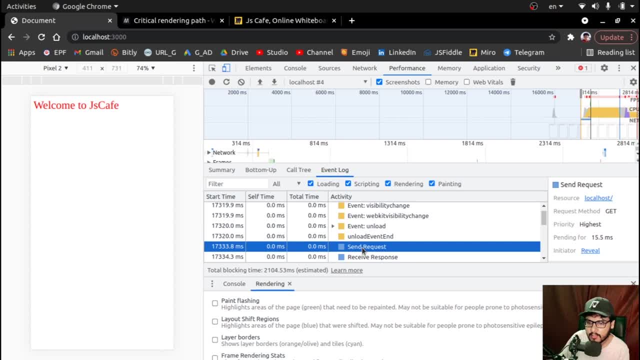 so you see that, uh, our, we initiated a send request. okay, on the localhost. i received a response. okay, i received the html response. and when i received html response- i- yeah, so i received html response- i finished the loading of this html and i started parsing my html. okay, so this is the parsing step. okay, this is what dom uh dong creation. 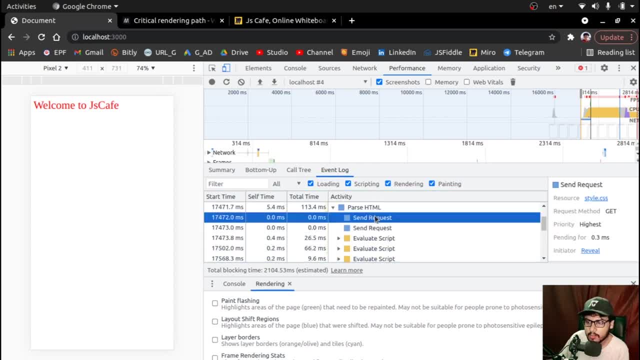 on creation. okay, in this parsing i send request to my stylecss file. i send request to my scriptjs file and i start evaluating my scripts and see here. i received a response from stylecss. i received the data from style. i started parsing my style sheets. okay, i finished the loading my style. 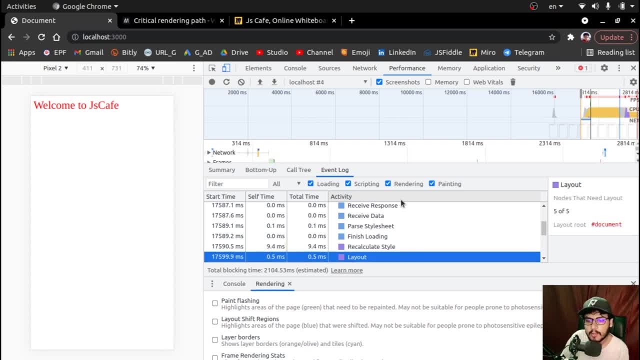 sheet. i recalculated my styles: okay, this is the layouting step i was discussing just about. okay, the layouting was happening and i updated the layer and see, this was the painting step. okay, the last step of the painting. and yeah, so, and this was like event load happening. uh, so this. 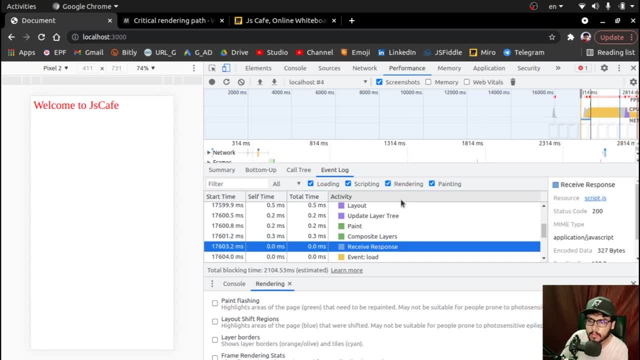 is the point, uh, where i got my script tag- okay, script. i received response of a script tag, i initiated an event load and i uh started uh other stuffs right. so this is, you know, this is what what the CRP- you know life cycle method- looks like, and I'll recommend you create your small dummies. HTML and CSS. 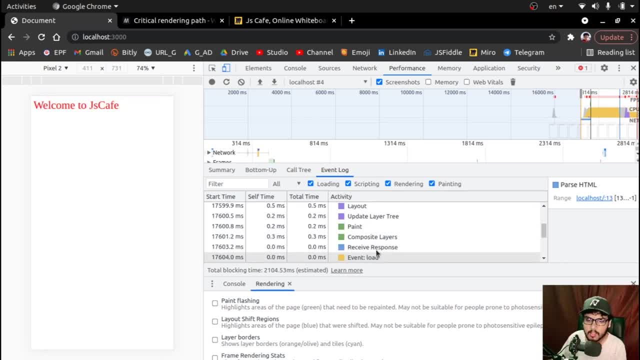 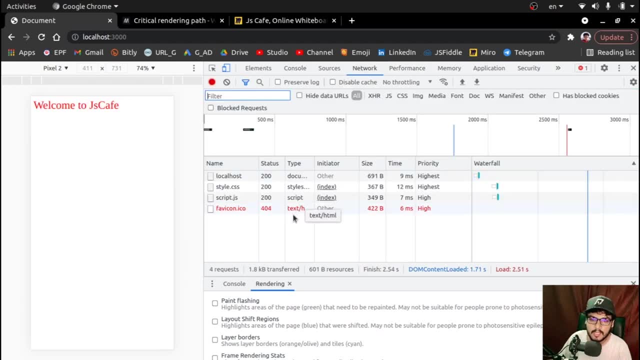 file and see how they look okay in this event log. yeah, so this was about the CRP and let me show you how these are, you know? yeah, so let me show you how CSS and JS are blocking actually your rendering and how things actually look when they. 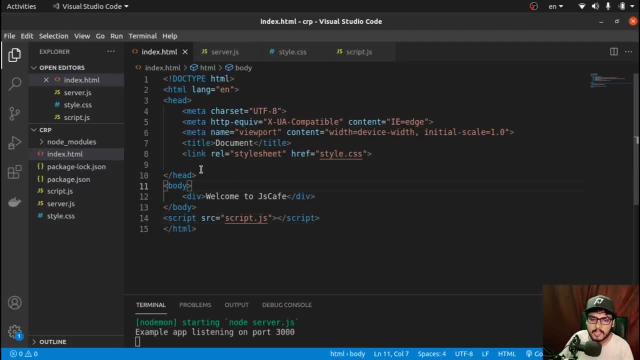 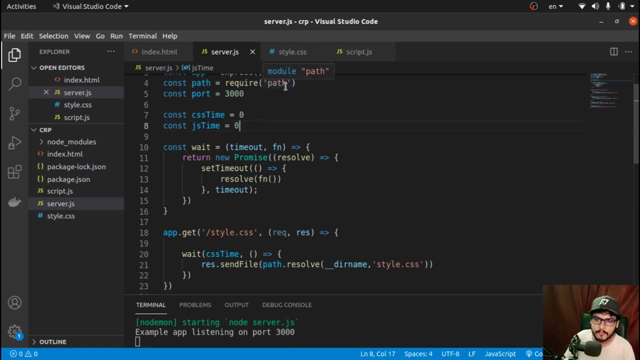 are loaded very slowly. so what I'll do is let me, for now, load this style sheet for a delay of 10 seconds. okay, so I'll add 10,000 milliseconds- okay, I like 10,000 milliseconds- and I load it for you and see what is happening. 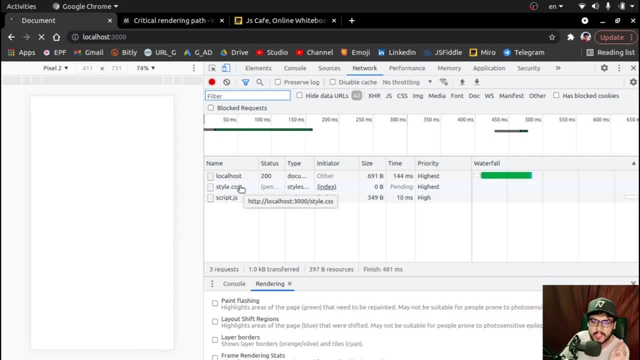 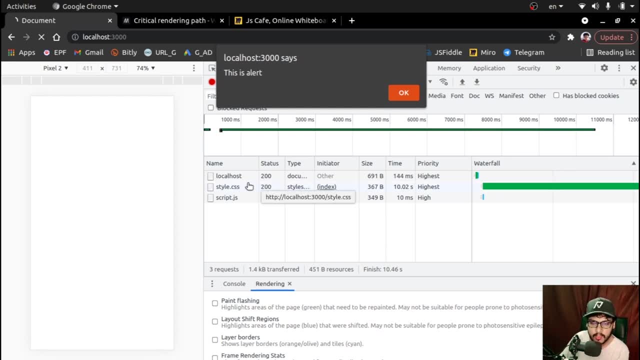 okay, so style sheet is still pending. I am NOT able to see anything. okay, after this style dot CSS was loaded again, I was able to execute this. you know JS, and after clicking ok, you can see that I am able to see this text over here. okay, so. 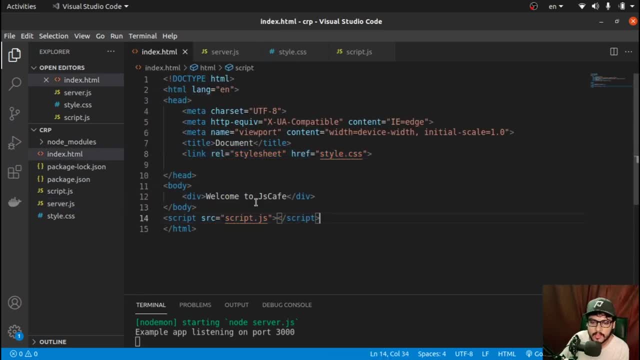 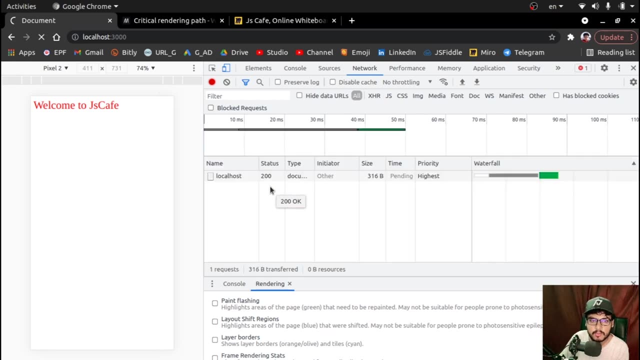 see this over here. see, this script is over here and we have this parsing right, so this was. let me show this again, if that was you know. so, okay, browser cleared the cache. now you see that we have this style or CSS over here. it is pending. we. 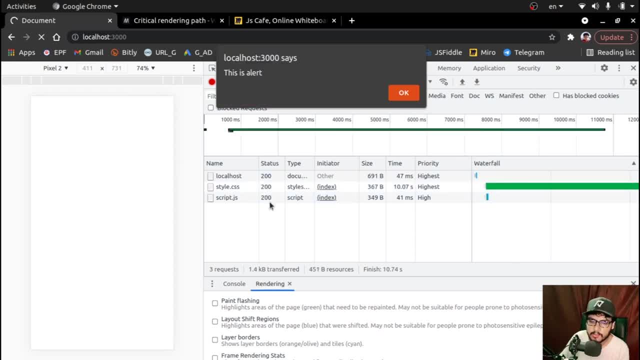 don't see any content once this style dot CSS is finished loading, our script was initiated and since this alert, you know, alert is also a blocking statement for us, so alert was again, is waiting for it, it to be, you know, clear. once we click OK, we are able to see this. welcome to GS cafe. now the point is that